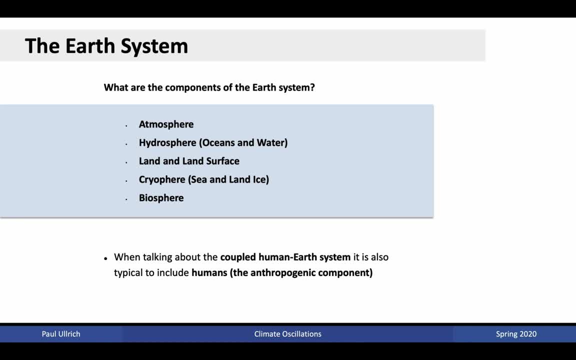 class that the major components of the Earth system are the atmosphere, the hydrosphere, the land and land surface, the cryosphere and the biosphere. Throughout this class, we've primarily focused on the first two reservoirs, that is, the atmosphere. 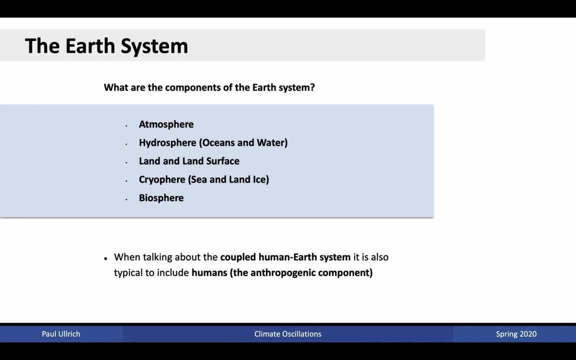 and the ocean. Hopefully, you've learned that these two are both very similar and very different from one another. The atmosphere is made of a compressible fluid and has its own set of dynamical equations that govern its motion. The ocean, on the other hand, is made up of a largely 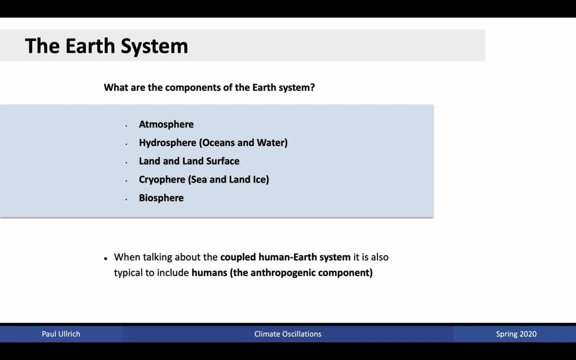 incompressible fluid and it is governed by parameters such as temperature and salinity. We have seen the atmosphere responds very rapidly to external forcing. The ocean, on the other hand, has very slow current velocities and tends to respond very slow, particularly at depth. So let's delve a little bit more into understanding. 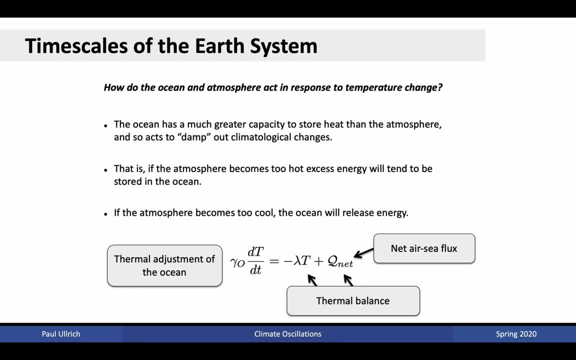 those time scales. Consider the following question: How do the ocean and atmosphere act in response to temperature change? Recall from our second lecture that the energy balance in the Earth system implies we must have no more energy leaving the system than we have energy coming in. However, we can exchange based on all the differentľe demonic patterns. 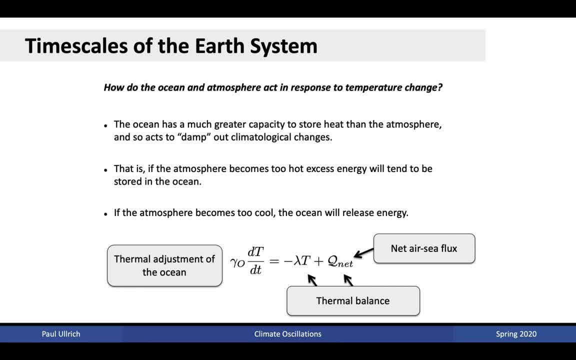 energy between the components of the Earth's system. Effects such as greenhouse gas emissions are responsible for redistributing that energy in the system, leading to near-surface cooling. We already know that the ocean has a much greater capacity to store heat than the atmosphere and consequently it has a 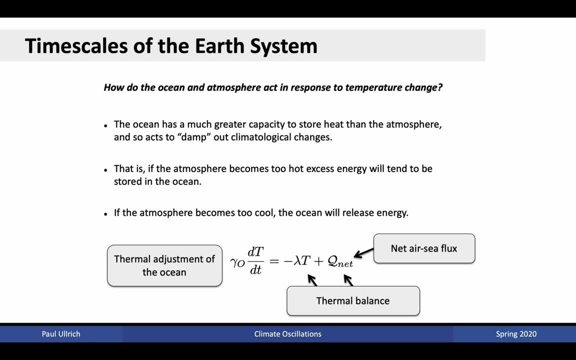 role of damping out climatological changes, That is, it tends to mitigate some of the effects from near-surface warming induced by, for instance, greenhouse gas emissions. So if the atmosphere becomes too hot, then excess energy will tend to be stored in the ocean In some sense, the ocean having its 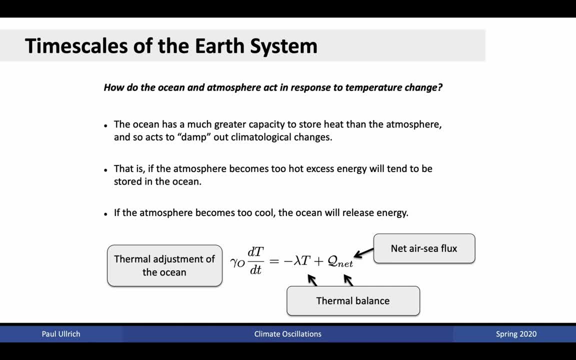 high heat capacity can act as a reservoir for that excess energy. Similarly, if the atmosphere becomes too cool, then the ocean will naturally release energy. One can describe this quantitatively using a simple thermal adjustment equation. On the left-hand side of this equation we represent the 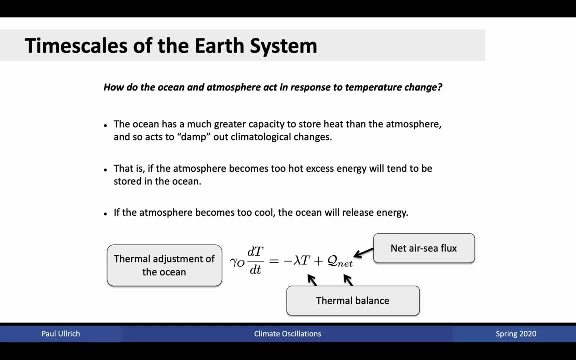 thermal adjustment of the ocean, which is the change in temperature of the ocean with respect to time. It has a constant of proportionality, which is the heat capacity of the particular region of the ocean that we're interested in. The change in temperature within this region is governed by two processes. One a 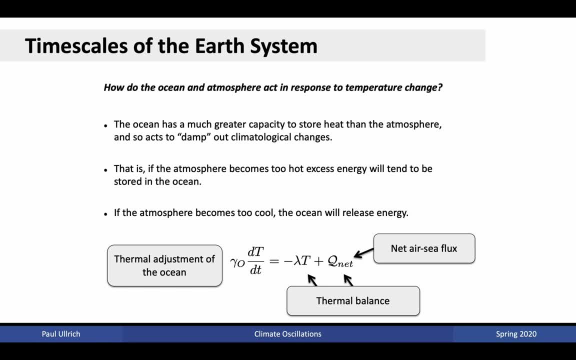 relaxation, which is representative of, for instance, radiative emission and latent heat fluxes from the ocean, That has a tendency, in order to draw down the temperature, That is balanced by an input of energy known as the net air-sea flux. 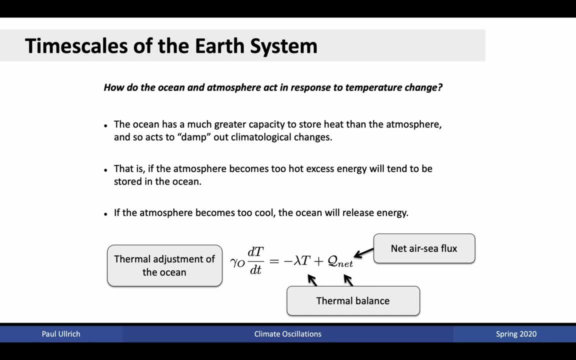 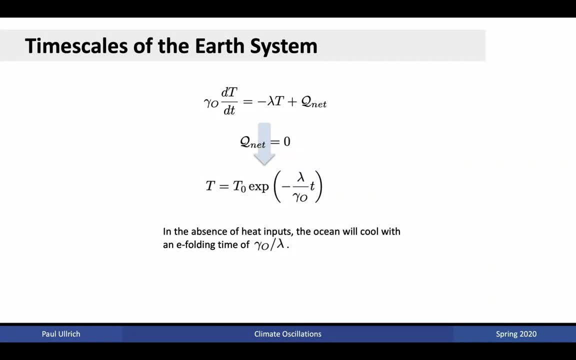 You'll notice that the change in temperature with respect to time is equal to zero when the thermal emission is balanced by the net air-sea flux. If we set the air-sea fluxes to zero, then the ocean will naturally cool over time. That is radiative emission and sensible and latent heat fluxes will. 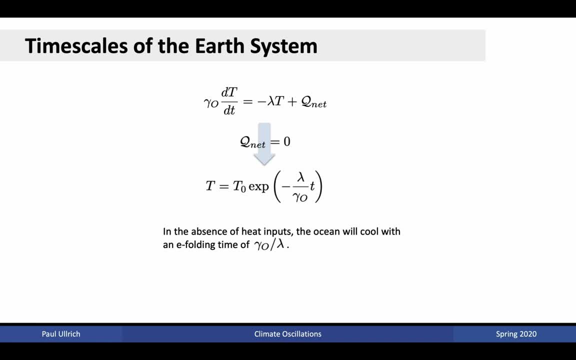 basically drive the temperature of the ocean down. If we solve this system for the case of q net equal to zero, we observe that the solution is simply a decaying exponential. The e-folding time associated with that exponential, that is the amount of time required for. 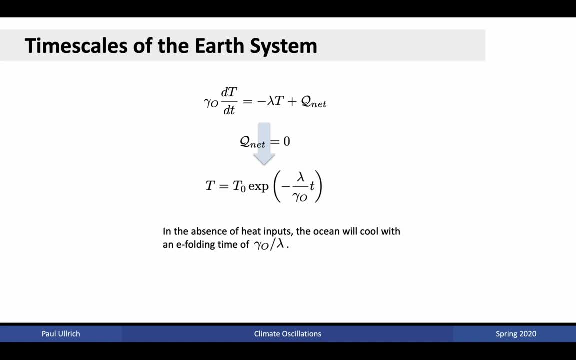 the temperature to drop by a factor of 1 over e will be given by gamma o divided by lambda. Thus, this factor, gamma o, governs the time scale of cooling associated with the ocean. Alright, let's try to calculate this gamma o. It is: 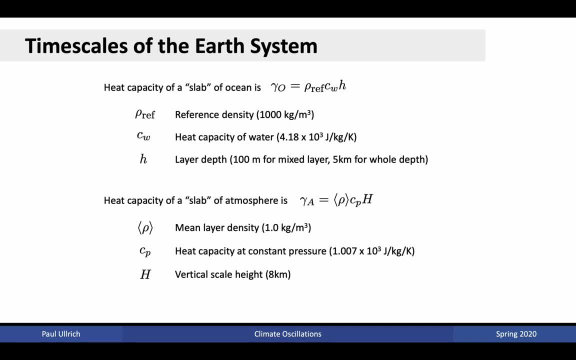 essentially a heat capacity of a slab of ocean. So gamma o is equal to the product of the density of the ocean water and the heat capacity of that water and the associated layer depth. Here the density is the reference density, taken as simply a thousand kilograms per meter cubed, and 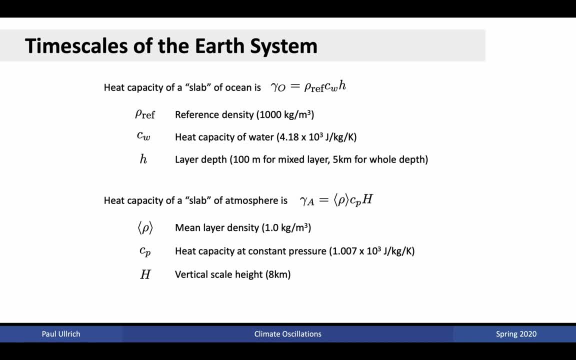 the heat capacity of water can be obtained from a lookup table. The layer depth depends on how much of the ocean you're considering in this analysis. If you only consider the mixed layer, which is in contact with the atmosphere because of turbulent processes over very short time scales, you would 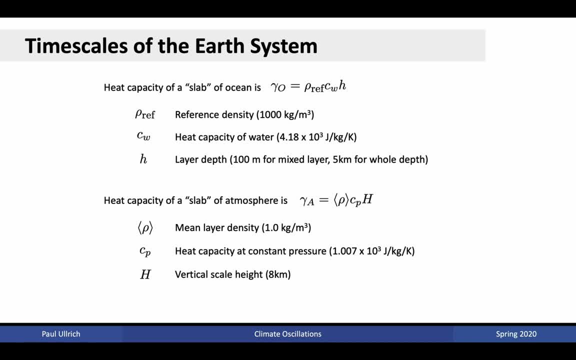 effectively choose a layer depth of about a hundred meters If you wanted to consider the whole ocean, so you want to consider, for instance, how long it takes the whole ocean to cool off- you would instead choose a layer depth of about five kilometers, Correspondingly the heat. 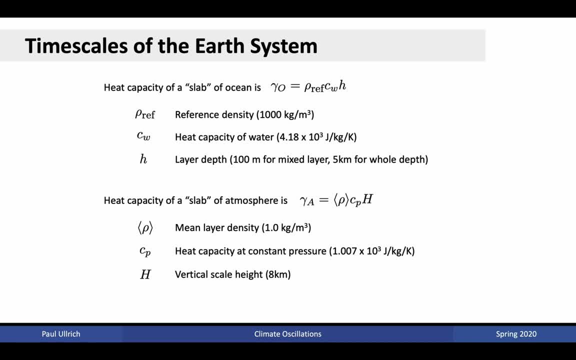 capacity of a slab of atmosphere can be denoted by gamma a and it's equal to a mean layer density times the heat capacity at constant pressure times. the vertical scale height of the atmosphere. All of these quantities we've had experience with previously in this class, The mean layer density, we're simply 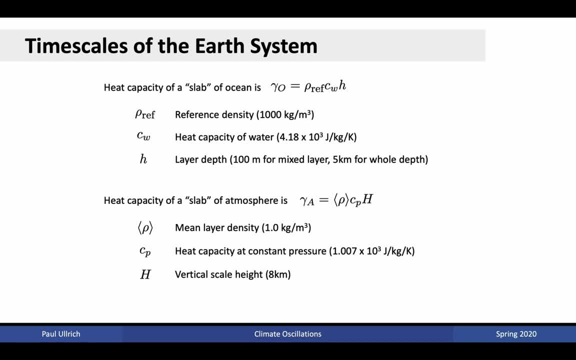 going to take to be the near-surface density. So we'll set that equal to one kilogram per meter cubed, acknowledging that it does drop substantially as one goes up in altitude. We can also choose the heat capacity at constant pressure to be 1.007 times 10 to the 3 joules per. 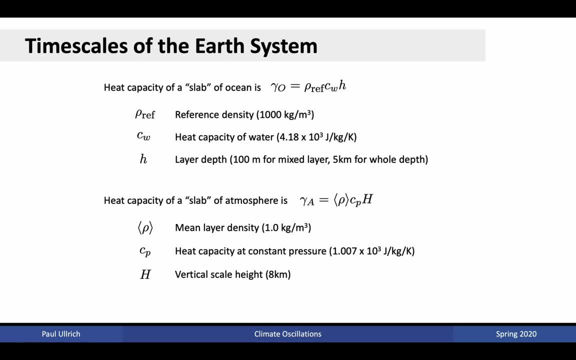 kilogram Kelvin, and we choose the vertical scale height, as we calculated earlier in this class, to be about 8 kilometers. So once you perform that calculation, you will then get approximations for the heat capacity of both the slab of ocean and the slab of atmosphere. 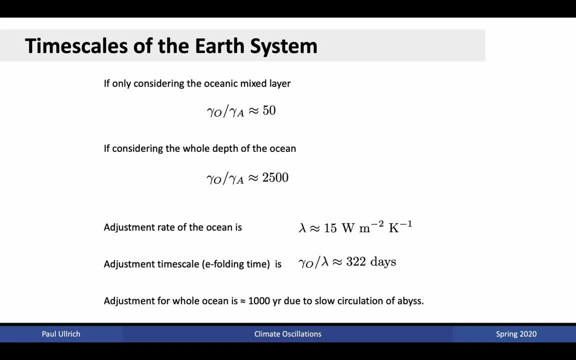 Comparing these two, one finds that, for instance, if you only consider the oceanic mixed layer, then you still get a heat capacity that's approximately 50 times that of the atmosphere. This demonstrates immediately that the ocean is a much greater reservoir of overall heat If you consider the whole depth of 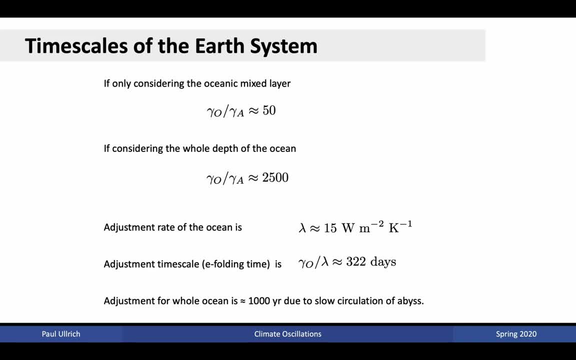 the ocean. the ratio of these two parameters is instead 2,500.. So, as you can see, the whole ocean itself essentially contains approximately 2,500 times as much energy as the troposphere of the Earth, If we use an adjustment rate of about 15 watts per meter squared per Kelvin, taken from 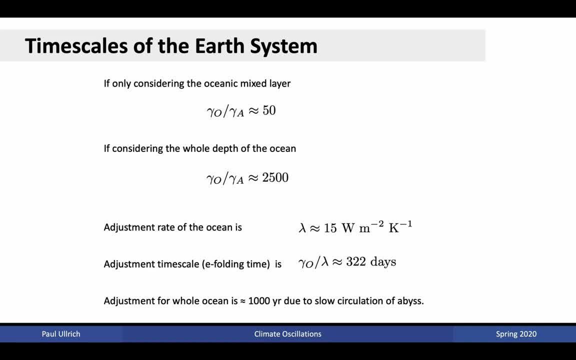 observations, then what we find is that the adjustment time scale for the mixed layer of the ocean is about 322 days. That is, cooling down the mixed layer of the ocean by a factor of 1 over e would take about 322 days. So obviously it's a. 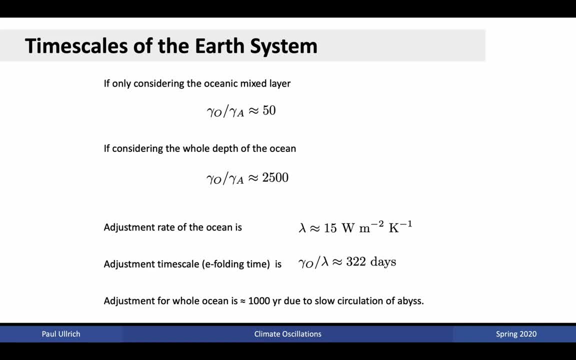 very slow process. overall, Adjusting the whole ocean takes about a thousand years. this is in part because the slow circulation that occurs in the abyssal layer as well. So we've already seen that the ocean is an excellent buffer of energy. How is this calculation different for the land surface? Well, we can perform. 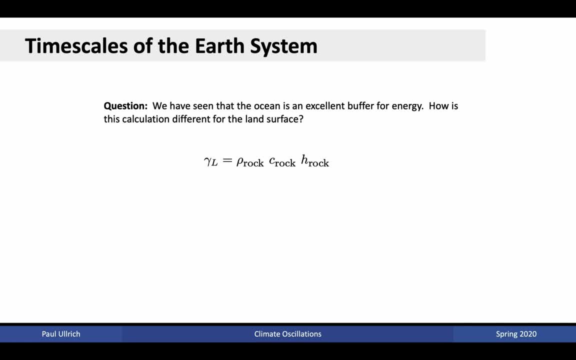 effectively an analogous calculation for land, here taking density of rock, heat capacity of rock and a height of rock, where the height is again taken to be approximately the region of the land surface that is in contact with the atmosphere. So how does this compare? Well, the density of rock will be a little bit. 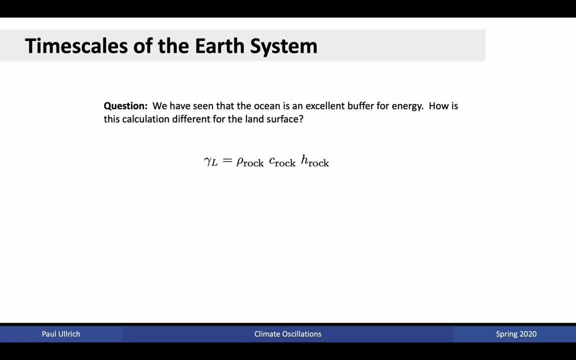 higher than in the ocean. certainly, The heat capacity is more or less proportional, but where we see the biggest change between the land surface and the ocean is really in this h parameter, Namely, there is not much of the land surface that is in contact with the atmosphere, whereas the ocean has a. 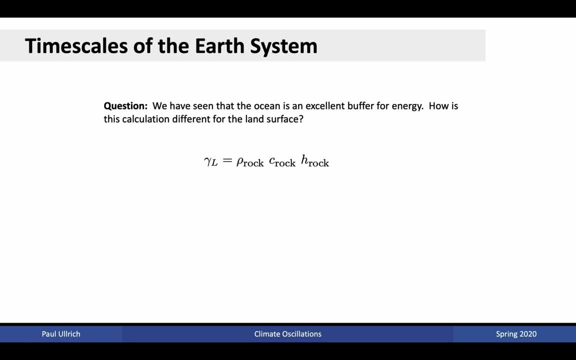 deep mixed layer and turbulent action that sustains that deep mixed layer. The land surface only has perhaps a 10 centimeters to a meter or so that can be considered to be in contact with the atmosphere. Consequently, this h parameter is much smaller in the land. 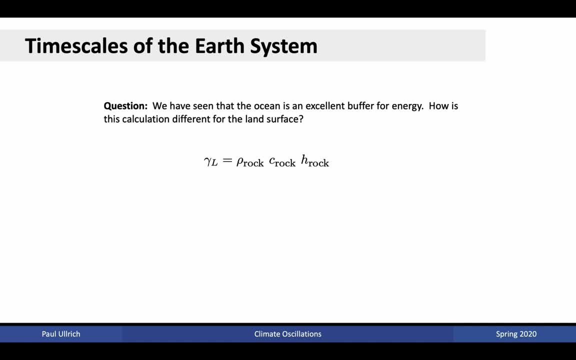 surface. So the heat capacity of the land surface is much smaller than in the ocean, and we see that the land surface then responds much more quickly to temperature changes than the ocean does. This is, then responsible for that inhomogeneity that we've discussed earlier in this class, Namely that the 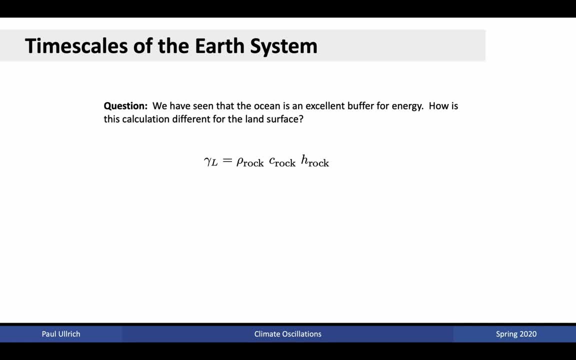 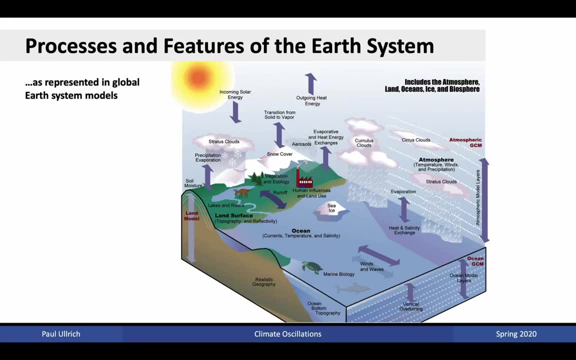 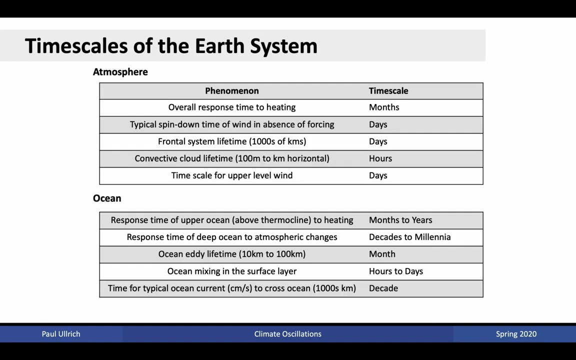 land surface tends to warm up and cool down much faster than the ocean. Besides thermal adjustment, there are many other processes and features of the Earth's system whose timescales we wish to understand. In the atmosphere, the overall response time to heating is typically on the timescale of months. The typical spin-down time of 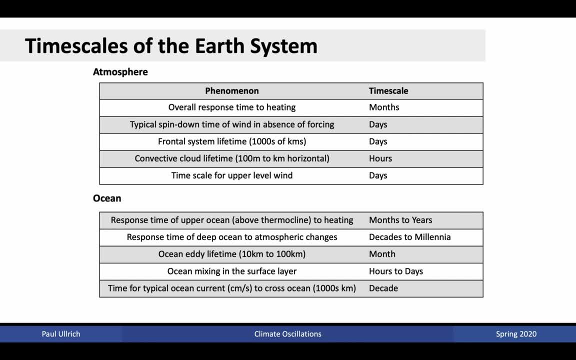 wind in the absence of forcing, is days. That is, if we were to shut down, for instance, external heating from the Sun, we would find that wind speeds would slowly reduce, and that would take only on the order of days for them to do so. 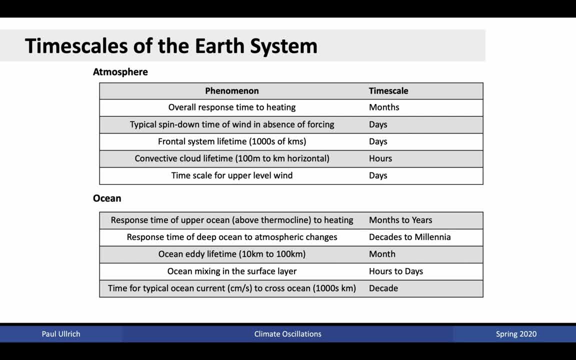 The frontal system lifetime, that is, these large-scale systems that propagate through the mid-latitudes- typically also have timescales of days associated with them. The convective cloud lifetime, which is typically on spatial scales of hundred meters to kilometers, only has hours associated with it, whereas the 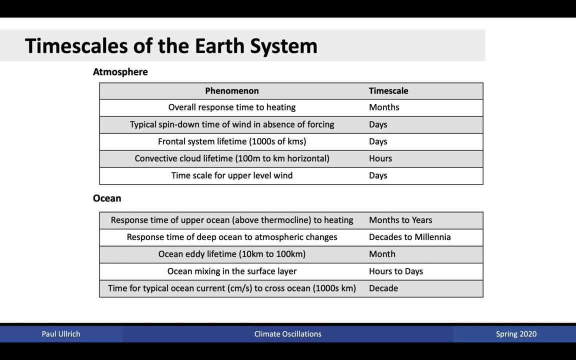 timescale of the upper-level systems, for instance, is only on the order of days. In the ocean, the response time of the upper ocean to heating is on the order of months to years, but the response time of the deep ocean to atmospheric changes can be on the order of decades to millennia. We've already 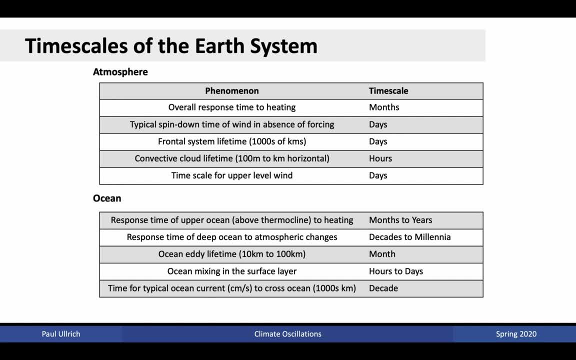 seen in our discussion of the oceans that CFCs, which are introduced in the atmosphere, take decades, to millennia, in order to propagate through the depths of the ocean. This is again due to the very slow circulations that occur in oceanic depths and the fact that one can't see a 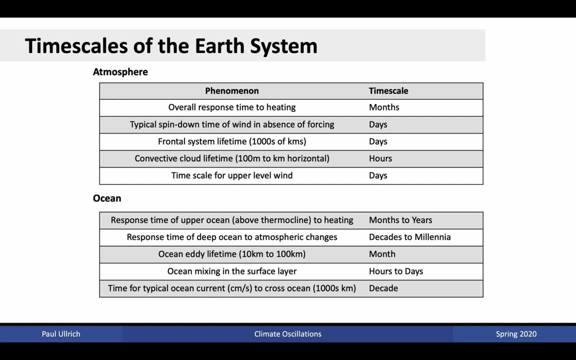 single cloud in the atmosphere and the fact that, once you get below the thermocline, there's very little influence from the atmosphere. The ocean eddy lifetime is on the order of months, ocean mixing in the surface layer is on the order of hours to days, and the time for a typical ocean current in order to 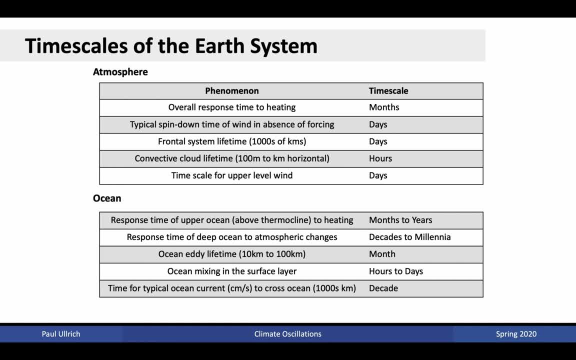 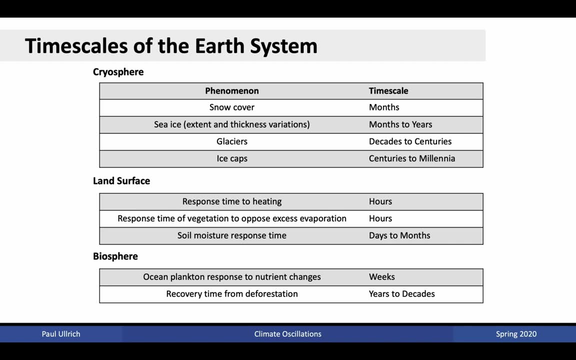 cross the ocean is on the order of a decade, So again, a very slow process. Contrasting these two, it is very clear that the ocean adjusts much more slowly than the atmosphere, The cryosphere, the land surface and the biosphere. We know that snow cover for 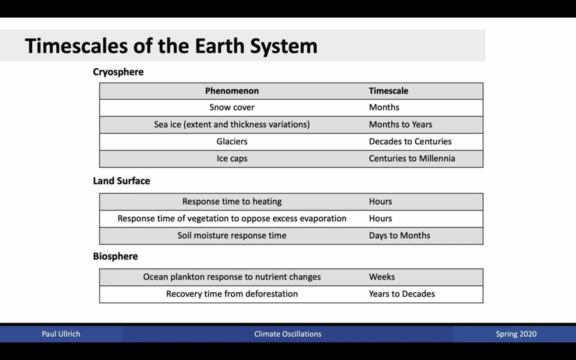 instance exists on the timescale of months, that is, it's roughly seasonal- and analogously with sea ice, Although with sea ice we can of course have buildups of sea ice that are associated with the longer processes. Glaciers take decades to. 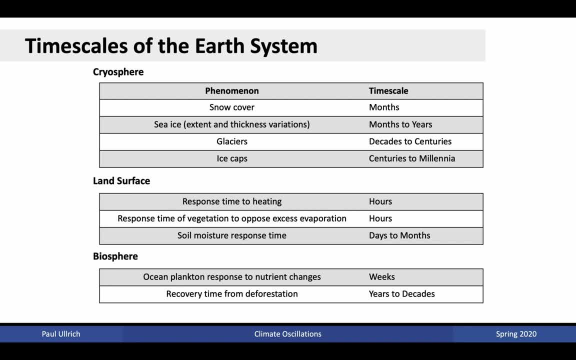 centuries in order to build up, but, as we've seen recently, they can be destroyed over much shorter time periods. if you crank up the thermostat. Ice caps, on the other hand, take centuries to millennia, that is, they accumulate over a very long period of time. However, again destruction. 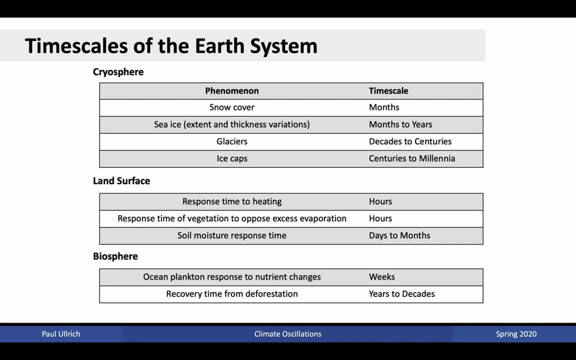 of these ice caps can occur over short time scales. The land surface, as we discussed earlier, has a very short response time to heating. It takes only on the order of hours for temperatures on the land surface to adjust changes in external forcing such as radiative forcing. Analogously, the response time to 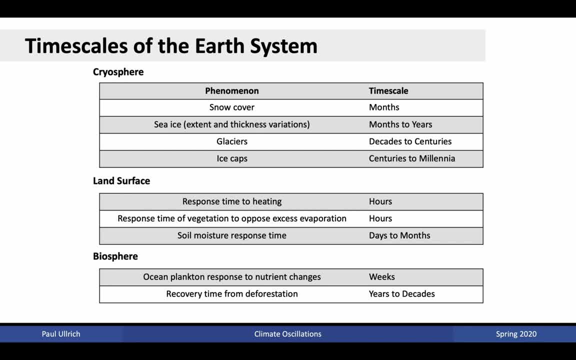 vegetation to oppose excess evaporation is also on the order of hours, and soil moisture response times are on the order of days to months. In the biosphere, ocean plankton's response to nutrient changes can take on the order of weeks, but recovery time from deforestation can take years to decades. 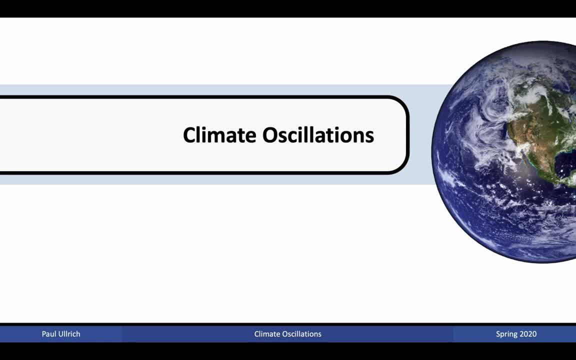 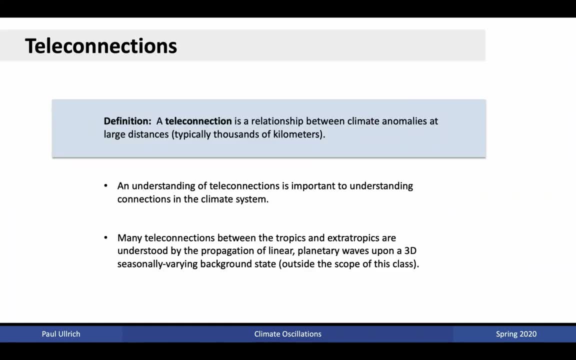 All right. now that we've talked about some of the timescales of the earth system, let's turn our attention to some of the large-scale climate oscillations that exist. Climate oscillations, which refers to periodic behavior within the global earth system, are closely connected with teleconnections. 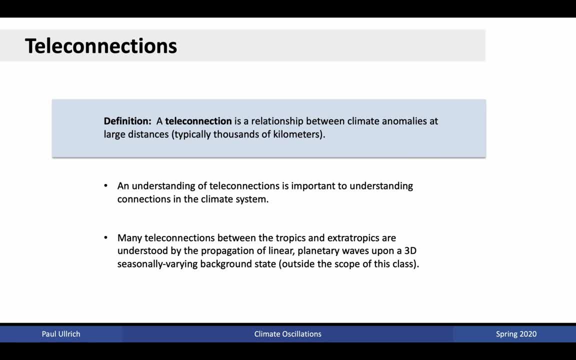 Teleconnections are relationships that occur between climate anomalies at large distances, typically on the order of thousands of kilometers. Major teleconnection centers of the world are known for propagating their influence globally and influencing the climate far away from those teleconnection centers. An understanding of these teleconnections is important to 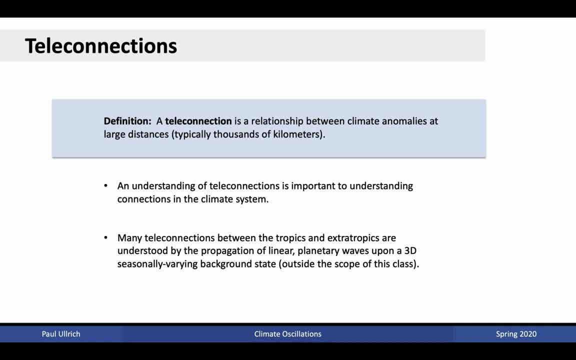 understanding connections within the climate system and propagation of information over large distances. Many of these teleconnections between the tropics and extratropics are under- stood primarily through the propagation of linear planetary waves upon a 3D seasonally varying background state. However, the investigation of the actual 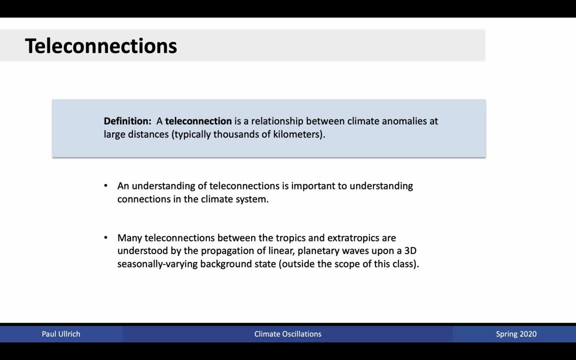 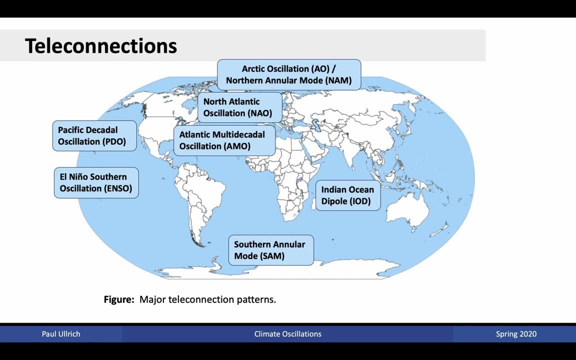 mechanisms by which these teleconnection centers propagate information globally is outside the scope of the current class. The teleconnection patterns that we'll be discussing in this class include the Arctic Oscillation, also known as the Northern Annular Mode, the North Atlantic Oscillation, the Atlantic 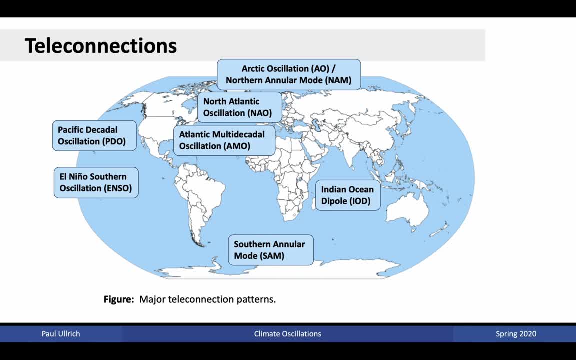 Multidecadal Oscillation, the Pacific Decadal Oscillation and the Indian Ocean Dipole. The El Niño Southern Oscillation is important enough that it deserves its own lecture, and so we'll discuss that in the next class. Alright, let's get started. So the Arctic Oscillation is the first. 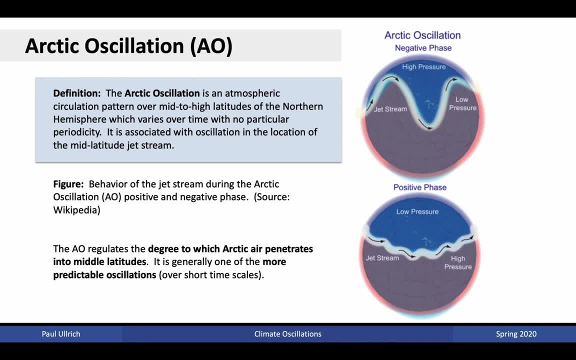 teleconnection pattern that we will be discussing. The Arctic Oscillation is an atmospheric circulation pattern over mid to high latitudes of the Northern Hemisphere which varies over time but has no particular periodicity associated with it. Its most obvious characteristic is the oscillation in the location of 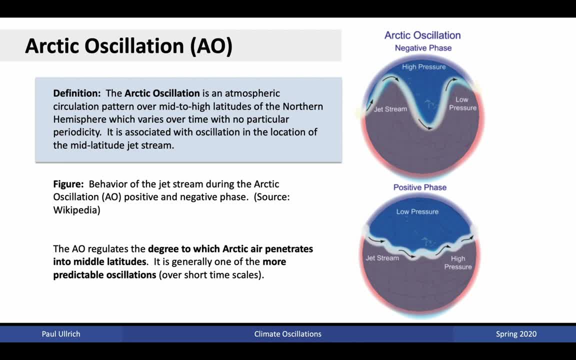 the mid-latitudinal jet stream. During the negative phase of the Arctic Oscillation, the mid-latitudinal jet stream tends to be more windy. During the positive phase, it tends to be more laminar or more straight, confined to a narrow band of latitudes. The Arctic Oscillation regulates the degree to. 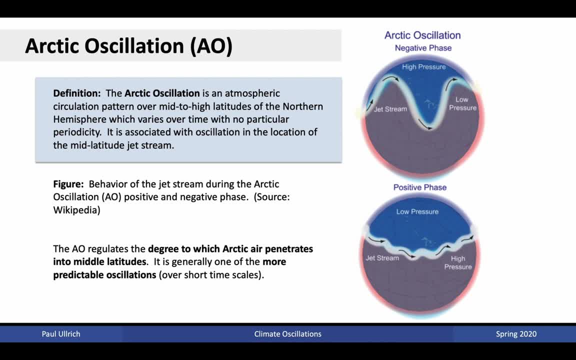 which Arctic air penetrates into the middle latitudes. It is generally one of the more predictable oscillations over shorter time scales and hence lends predictability over periods longer than the typical forecast window of seven to ten days. During the negative phase, we have a tendency for 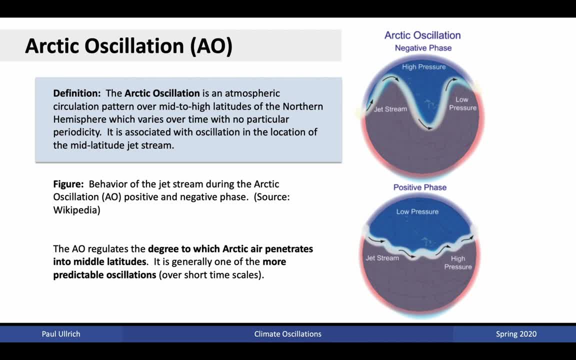 more Arctic air to penetrate farther south. Consequently, this can lead to cold conditions in more southern latitudes than they would appear. typically. During the positive phase, we have more isolation of that Arctic air. Typically, this is associated with larger temperature gradients around the location of the jet stream, but also a tendency for that Arctic air to not. 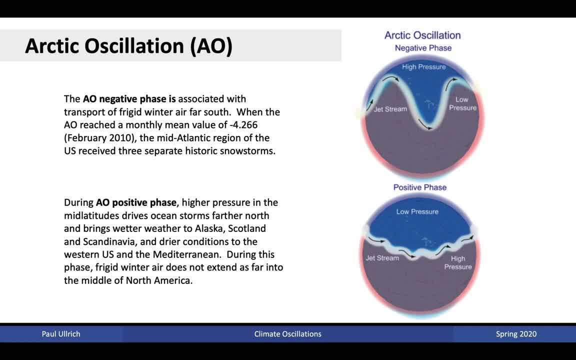 penetrate into farther southern latitudes. The negative phase in particular is associated with the transport of this frigid air far south In February 2010, when the Arctic Oscillation reached its index value of minus 4.266, which was the record for the time, the US received. 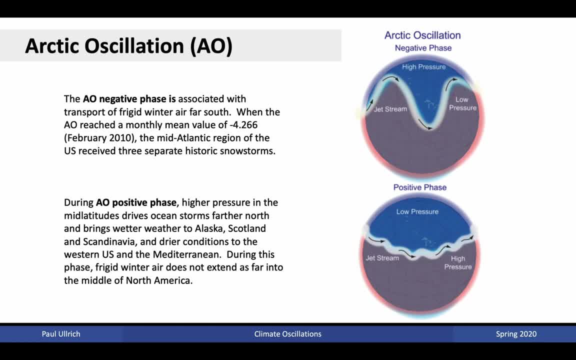 three separate historic snowstorms because of the transport of this cold air. During the positive phase, the higher pressure in the mid-latitudes tends to drive ocean storms farther north and tends to bring wetter weather to Alaska and Scandinavia, as well as drier conditions to the western US and the 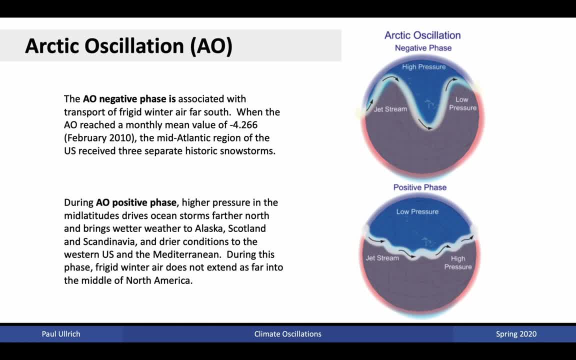 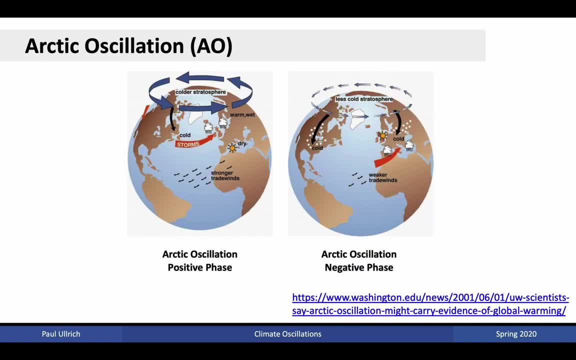 Mediterranean. During this phase, frigid winter air does not extend far south into middle America and tends to be isolated within the Arctic region. Here are some of the meteorological patterns that are associated with the Arctic Oscillation. Again, during the positive phase, we have a very strong jet that 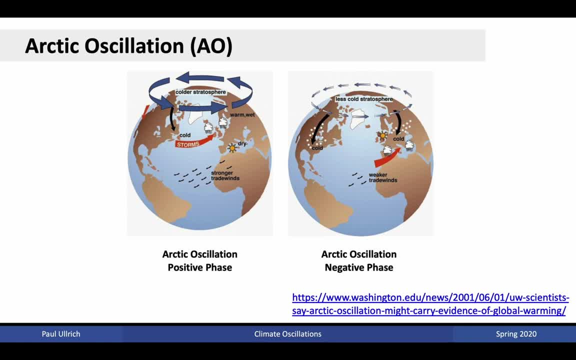 tends to isolate cold Arctic air in the higher latitudes. This is then associated with a stronger storm track and, consequently, a higher temperature. This is then associated with a stronger storm track and, consequently, a higher temperature. This is then associated with a stronger storm track and consequently, 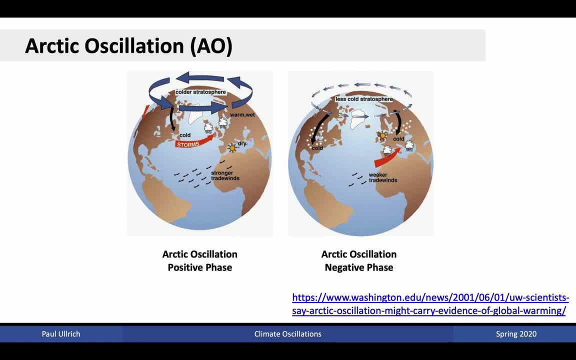 storms that propagate across the Atlantic, bringing warm and wet conditions to northern Europe. Because the storms are also farther north, southern Europe tends to be drier. This pattern is also typically associated with stronger trade winds During the negative phase of the Oscillation we have. 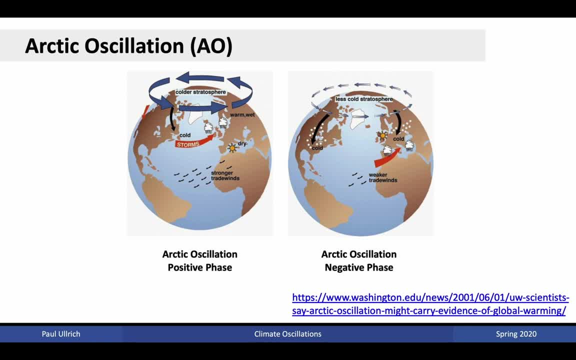 a very windy yet weak jet stream. Consequently, there's more opportunity for cold Arctic air to penetrate southwards, and that brings cold conditions to both middle America and to Central Europe. However, because of the weaker trade winds, we also then have typically storms that can 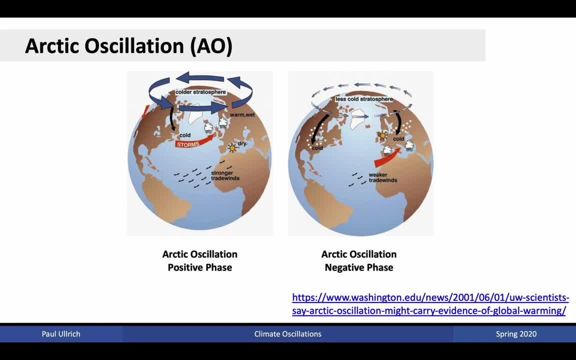 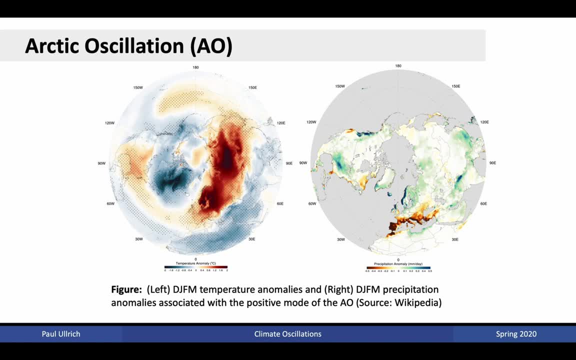 propagate into southern Europe, bringing wetter conditions through that region. On the left-hand side of this plot we see the temperature anomalies associated with the Arctic Oscillation, and on the right we see the precipitation anomalies. Note that these plots are both made looking directly down on the north pole. What we 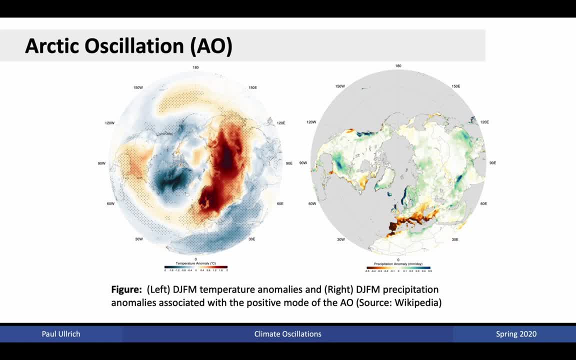 see in the temperature anomaly plot is that during the positive phase of this Oscillation we have colder conditions, isolated in the Arctic That is. we see cold weather in Greenland and in northern Quebec in Canada, but it's associated with warmer conditions farther south. So much of Europe, central Russia. 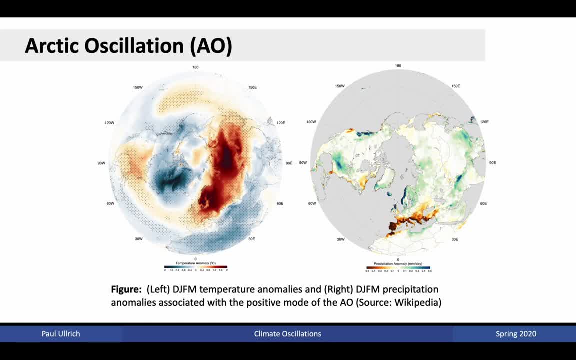 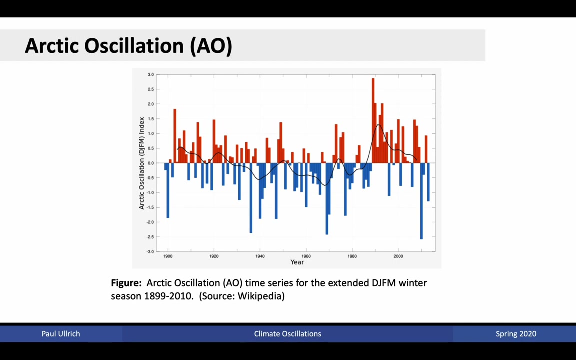 and the lower latitudes of the continental United States experience warmer conditions during the positive phase of the Arctic Oscillation. The precipitation fields associated with the Arctic Oscillation indicate wetter conditions through middle America but drier conditions through southern Europe during this time. Here's a time series of the extended December, January, February. 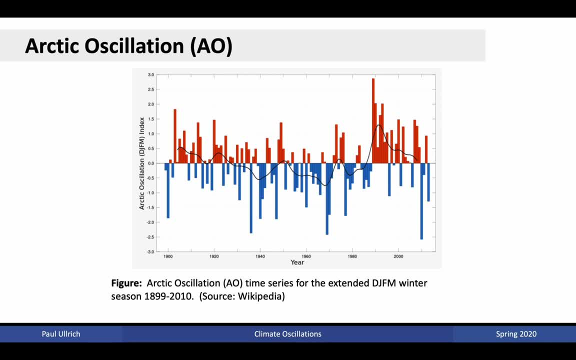 March, winter season. showing the Arctic Oscillation indices. Red in this plot corresponds to positive phases of the Arctic Oscillation and blue corresponds to negative phases. As we can see, there's no obvious trend over this short time period. However, more recently we have seen more instances of positive phase Arctic Oscillation. 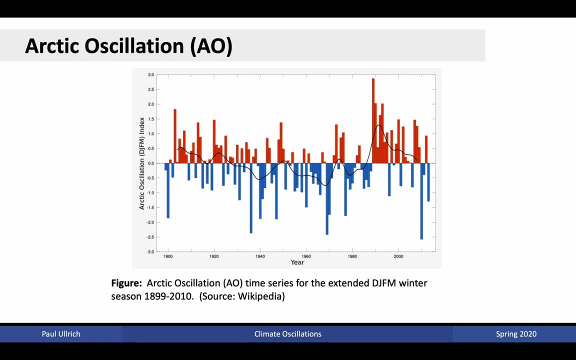 However, we also see very extreme negative phase Arctic Oscillation In particular. the most extreme negative Arctic Oscillation value on record occurred in 2010.. At this most negative monthly mean value, this was associated with three separate historic snowstorms, as mentioned earlier. 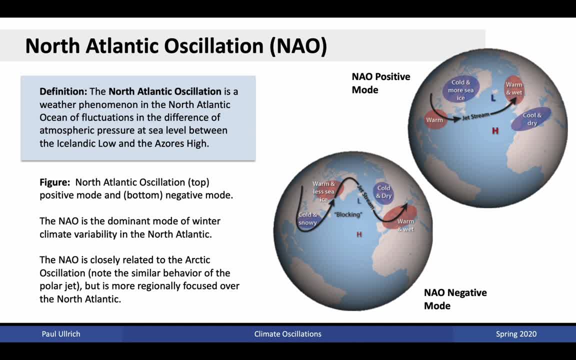 All right, let's turn our attention to the North Atlantic Oscillation. The North Atlantic Oscillation is a very common phenomenon in the Arctic. It's a very common phenomenon in the Arctic. The Arctic Oscillation is very closely connected with the Arctic Oscillation and is also associated. 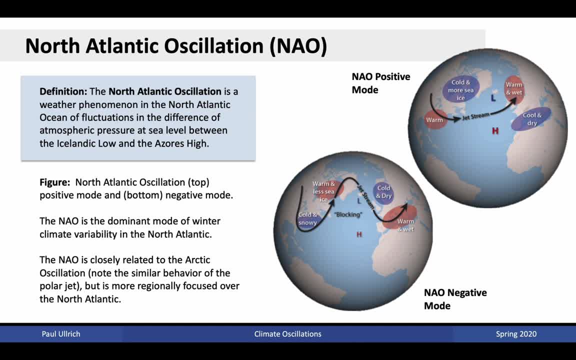 with the windiness of the jet stream. The North Atlantic Oscillation is a weather phenomenon in the North Atlantic Ocean of fluctuations in the differences between atmospheric pressure at sea level between the Icelandic low and the Azores high. Obviously, since it's associated with these. 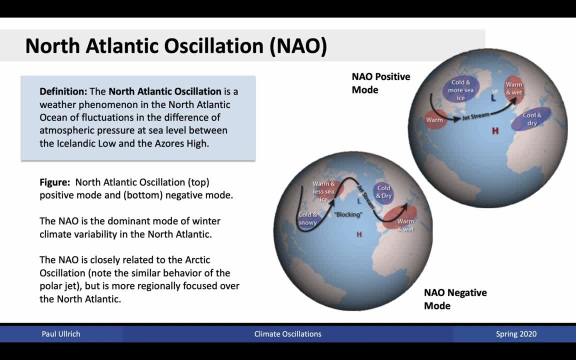 fluctuations in sea level pressure. it is also closely connected with the jet stream via geostrophic flow relationships. The North Atlantic Oscillation is a very common phenomenon in the Arctic, particularly in southern apartment areas, and these situations can be expected to translate into Fitland Cliffs For adopted weather. it is easily understandable that North Atlantic 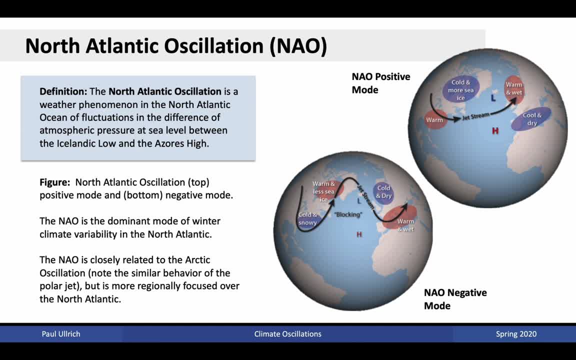 is a cross- plupart ideal climate. At a number of points this relationship is very observe, since above the horizon offers aеро-hображable map of the Arctic Ocean. as you can see here, At average Arcticução is as exposed to surface waves as possible, but at the moment we are in the Arctic Ocean. 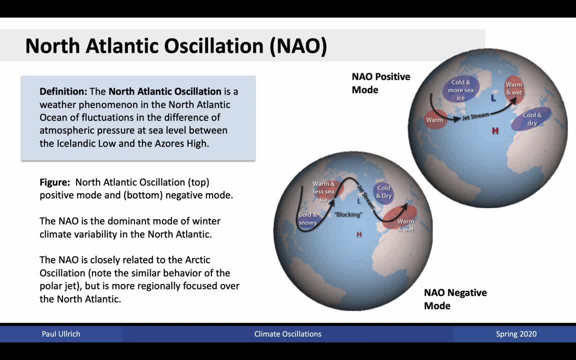 as the orada and the North Atlantic options are an Academy of yourيع. accept你看 In both ways сил의. as cool and dry conditions in southern Europe. These also correspond to warm conditions in the southeast of the US and warm and wet conditions through northern Europe. The negative phase of 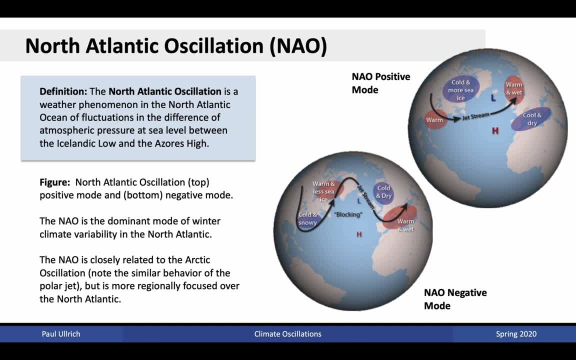 this mode is associated with warm conditions in northern Canada, as well as less sea ice, and is associated with cold and snowy conditions along the eastern seaboard of the continental US. It's also associated with cool and dry conditions in northern Europe and warm and wet conditions. 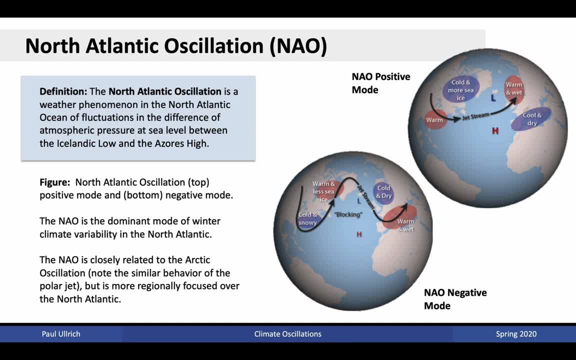 in southern Europe. The NAO is again closely related to the Arctic Oscillation but tends to be more regionally focused. If you look at the sea level pressure anomalies associated with both these patterns, they are closely related but still not quite on top of each other. 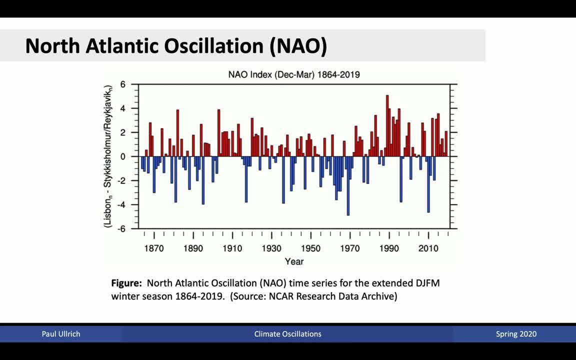 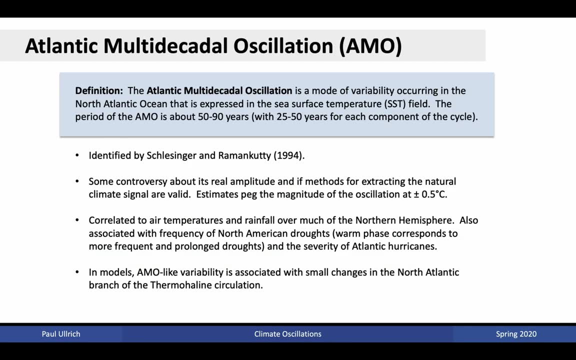 Here's the NAO index time series for the extended December, January, February, March, winter season extending back to 1864.. As we can see, it varies between both positive mode and negative mode. All right, the third form of oscillation that we'll be looking at is the Atlantic Multidecadal. 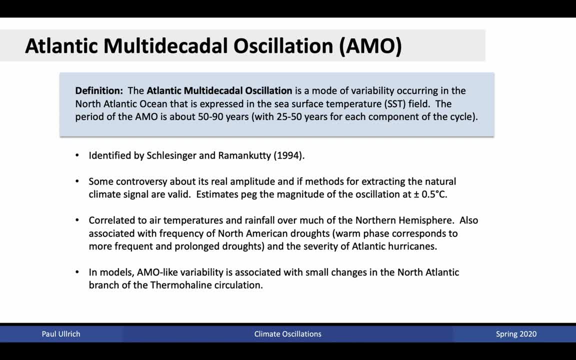 Oscillation. This is a mode of variability occurring in the North Atlantic Ocean that is expressed in the sea surface temperature field. The period of the Atlantic Multidecadal Oscillation is about 50 to 90 years, with about 25 to 50 years associated with each component. 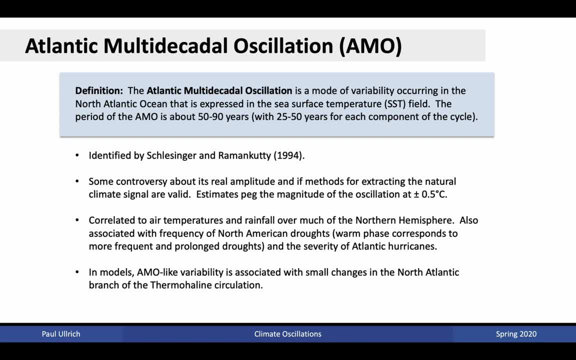 of the cycle, That is, typically it's in a positive phase, or leaning towards a positive phase for about 25 to 50 years and then switches into a negative phase. This pattern was originally identified by Schlesinger and Ramankutty in 1994.. However, 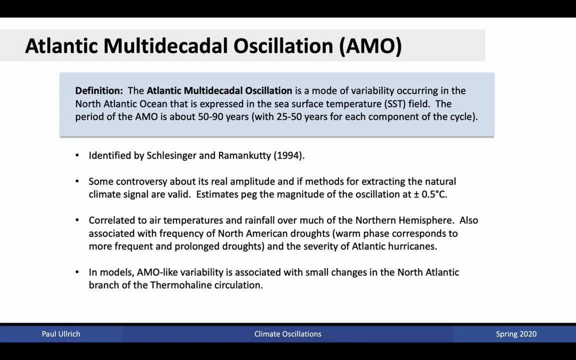 there's some controversy about its real amplitude and if the methods for extracting the natural climate signal are valid. Nonetheless, the estimates peg the magnitude of this oscillation at about half a degree Celsius. This oscillation is strongly correlated with air temperatures and rainfall over much of the northern hemisphere. As one would expect, this Multidecadal Oscillation 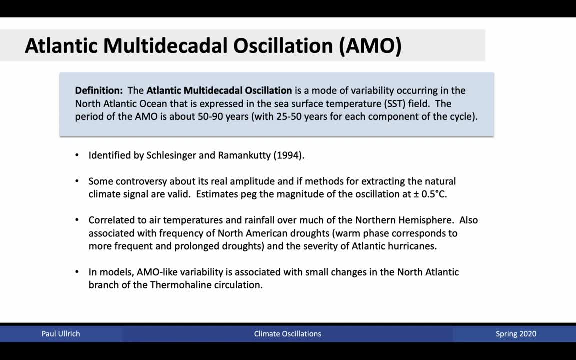 affects the northern Atlantic sea surface temperatures. The warmer temperatures can then impact the warming of the northern hemisphere. These warmer conditions can then impact evaporation, which can impact the amount of moisture present within the air. This Multidecadal Oscillation is also associated with the frequency of North 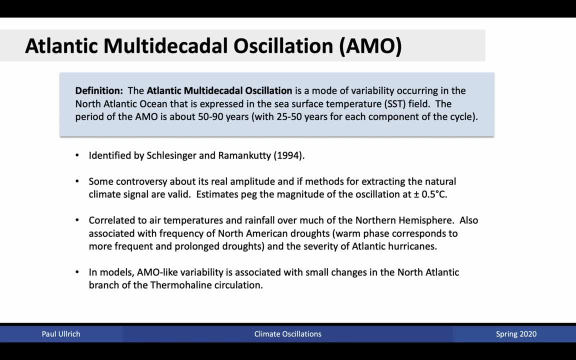 American droughts, with the warm phase corresponding to more frequent and prolonged droughts, as well as the severity of Atlantic hurricanes. Typically, warmer Atlantic waters are associated with more intense hurricanes. In models, this AMO-like variability is often seen in the North Atlantic Ocean In the 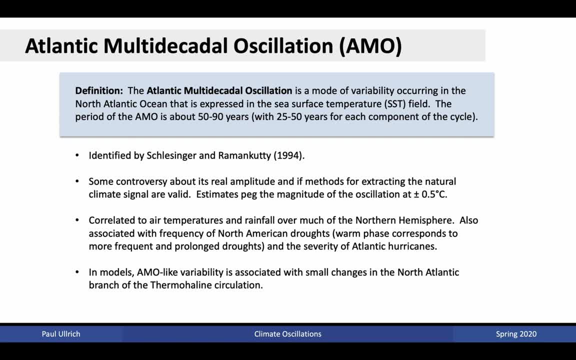 models, this AMO-like variability is often seen in the North Atlantic Ocean. In the models, this AMO-like variability is often seen in the North Atlantic Ocean. In the models, this AMO-like variability is associated with small changes in the North Atlantic branch of the thermohaline circulation. 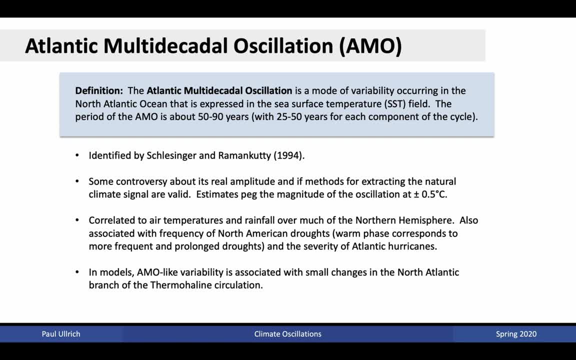 Recall from last time we discussed how the thermohaline is responsible for bringing warm waters into the North Atlantic, as well as being responsible for driving things like sea ice extent. The AMO, then, is closely connected to the variations that occur within the thermohaline. 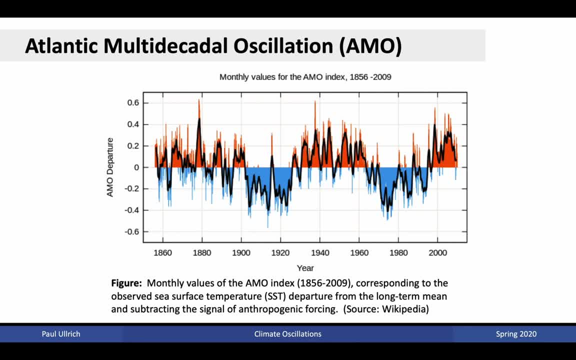 Here are monthly values of the Atlantic Multidecadal Oscillation Index, showing positive phase and negative phase. The departures here correspond to sea surface temperature departures. so positive values are warmer conditions in the North Atlantic and cooler conditions in the North Atlantic. 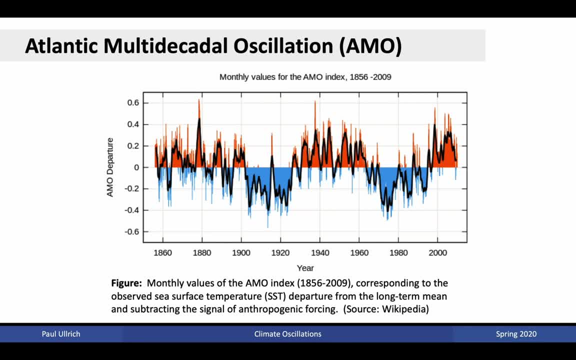 This is obtained by taking observed sea surface temperature records and subtracting the long-term mean value as well as the signal that comes from anthropogenic forcing, which would naturally give an upward trend associated with this profile. As we can see, we have extended periods of positive. 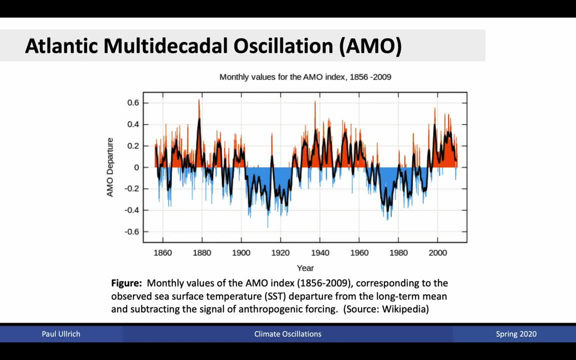 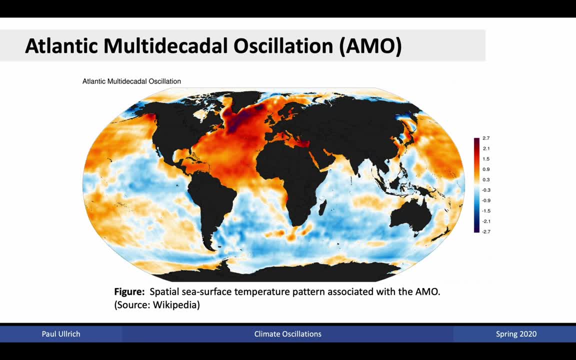 values of the AMO, as well as extended periods of negative values. Here is the pattern associated with the Atlantic Multidecadal Oscillation. Again, during the positive or warm phase, we see much warmer oceanic conditions that extend far north to the Labrador Sea and to Greenland, whereas during the cooler phase, 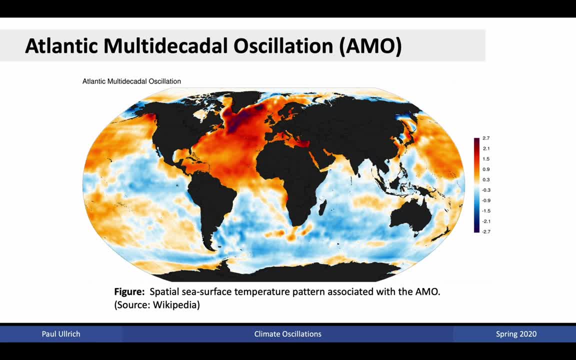 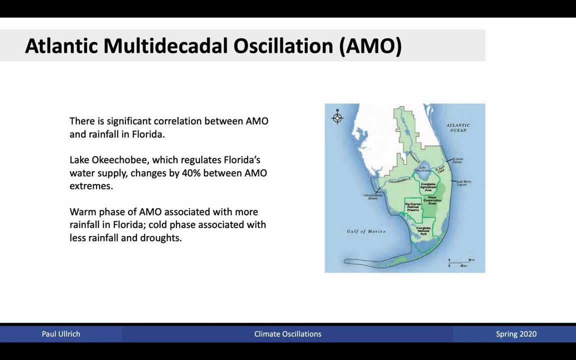 we effectively get the negative of this signal, that is, we have cooler temperatures throughout the North Atlantic. It's known that there is a significant correlation between the Atlantic Multidecadal Oscillation and rainfall. in Florida, As we know, during the warm phase we have more evaporation from the ocean surface, as 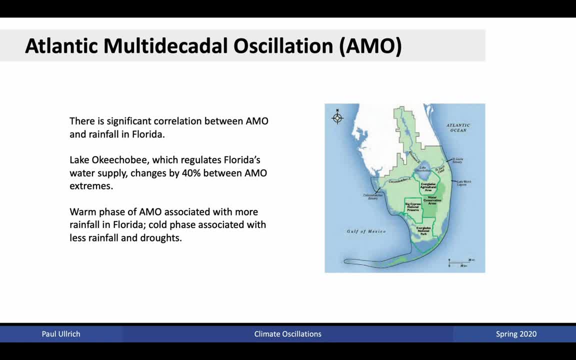 well as warmer near-surface airs. Consequently, the atmosphere can hold more moisture and so will have a tendency to produce more precipitation. Since the climate of Florida is so strongly connected to that of the Atlantic Ocean, water resources in Florida are largely impacted by changes in sea surface temperatures within 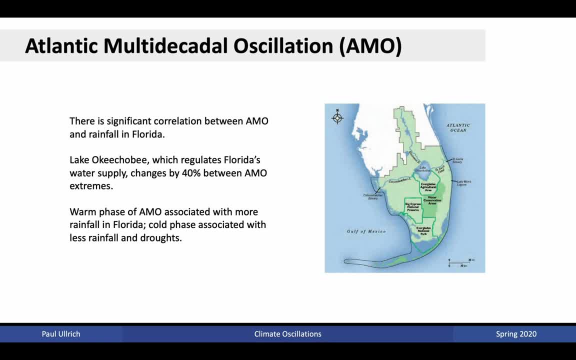 this region. It is known that the lake levels in Lake Okeechobee can change by 40% between AMO extremes. That is, during the warm phase of the AMO we typically have much more precipitation and consequently a higher level in the lake. 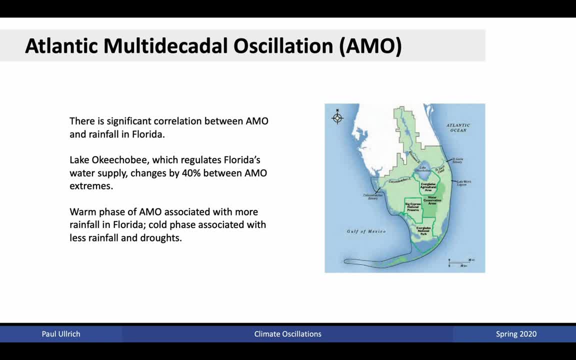 During the cold phase. on the other hand, this is associated with less rainfall and more frequent droughts within the region. However, the warm phase also comes with more tropical cyclones, because those warmer ocean waters are again driving up the intensity of those storms. 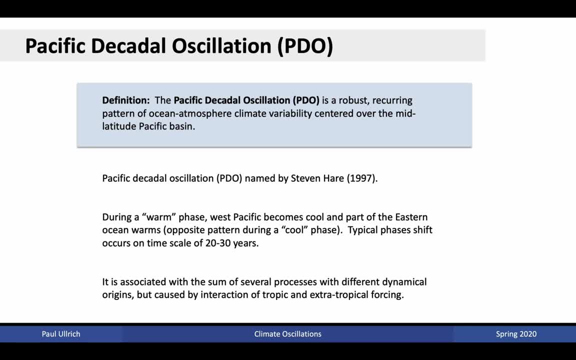 In the Pacific Ocean there is a corresponding partner to the AMO known as the Pacific Decadal Oscillation. This is a robust recurring pattern of ocean-atmosphere climate variability centered over the mid-latitude Pacific Basin. This was originally named by Stephen Hare in 1997.. 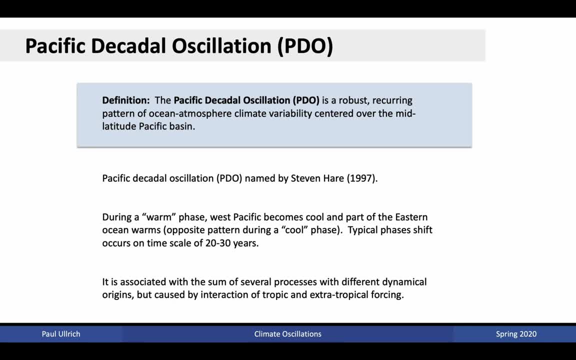 During the warm phase of the Pacific Decadal Oscillation, the West Pacific cools and part of the Eastern Ocean warms. The opposite pattern shows up during the cool phase. The PDO pattern can actually be seen through much of the Pacific Typical phase. shifts in the PDO typically occur on a timescale of 20-30 years. 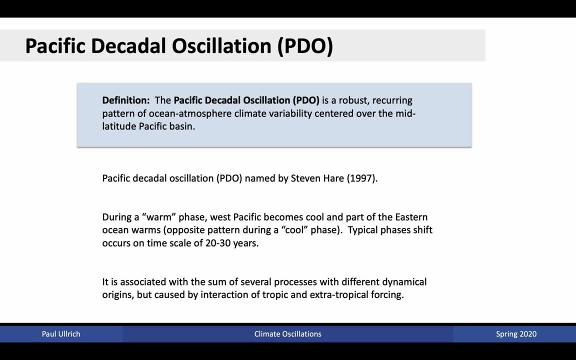 That is analogous to the Atlantic Multi-Decadal Oscillation. the PDO tends to exist within a certain phase pattern, for 20-30 years, before flipping to its other mode. The PDO is associated with the sum of several processes that have different dynamical origins. 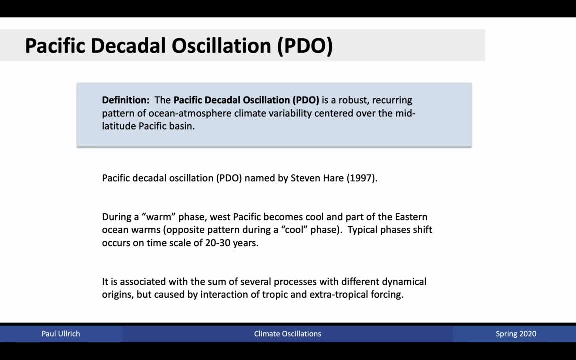 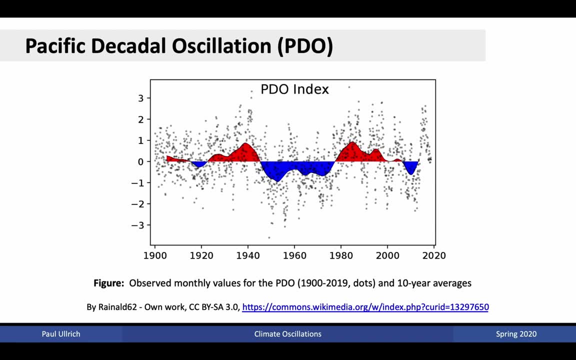 but is primarily caused by the interaction of both tropical and ocean-atmosphere climate variations. Here's the Pacific Decadal Oscillation index, observed back to 1900.. Here we again see positive and negative modes associated with the PDO, with a strong positive. 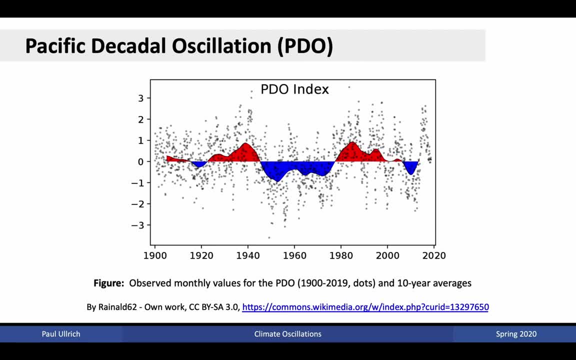 period occurring between 1920 and approximately 1945, followed by a negative mode period and then, in the 1980s, picking up again in the positive mode. Recently, we've seen oscillations as well as the mode shifts between negative to positive. 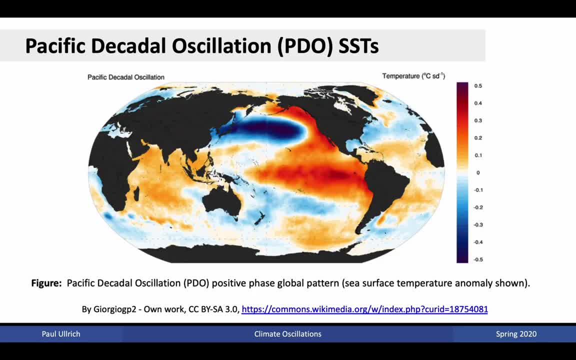 Here are the sea surface temperatures associated with the Pacific Decadal Oscillation pattern. This is the positive mode, that is, it's associated with cooler temperatures in the western north Pacific and warmer temperatures in the coastal Pacific. This pattern actually looks quite analogous to the El Niño mode, that is, it's associated 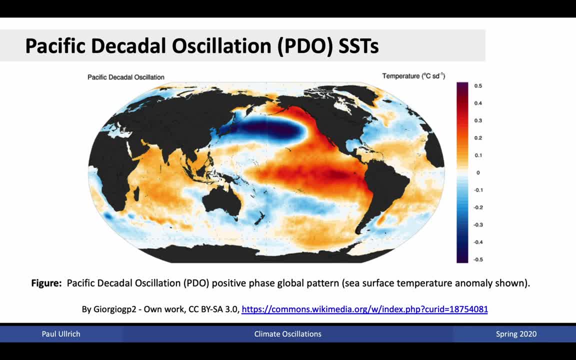 with warmer temperatures in the eastern tropical Pacific as well. Here are the time scales. The time scale, though, is based on the Pacific Decadal Oscillation pattern. The time scale is not unique to the Pacific Decadal Oscillation pattern because in the 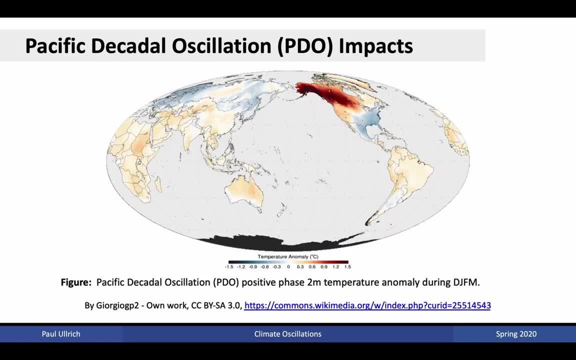 decadal oscillation are much longer than those of El Niño. Impacts of Pacific decadal oscillation include both temperature and precipitation impacts. Here we see the impact on the two meter temperature or near surface temperature through the northern hemisphere In Alaska, along the west coast of Canada. 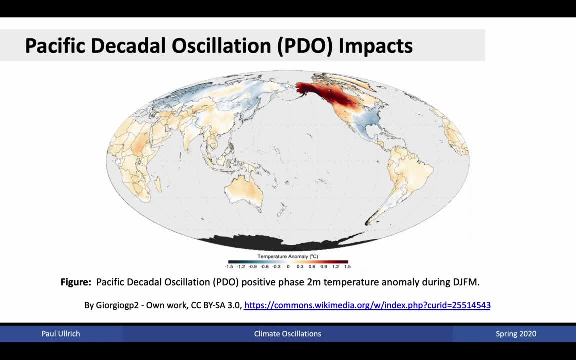 and the west coast of the continental US. the positive phase of the PDO is associated with much warmer temperatures in these coastal regions. On the other side of the Pacific, we see cooler temperatures. This is simply because of regional forcing, because of this temperature shift in the Pacific Ocean. 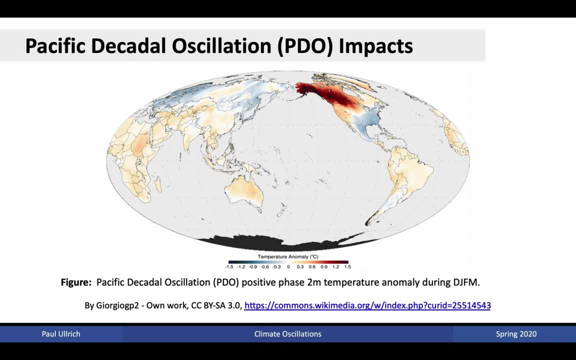 waters. However, there is a broader extent associated with these impacts as well. We see weak forcing that extends over much of the globe associated with the positive mode. The negative mode is analogous except with the sign flipped. Here are the precipitation patterns associated with the Pacific decadal. 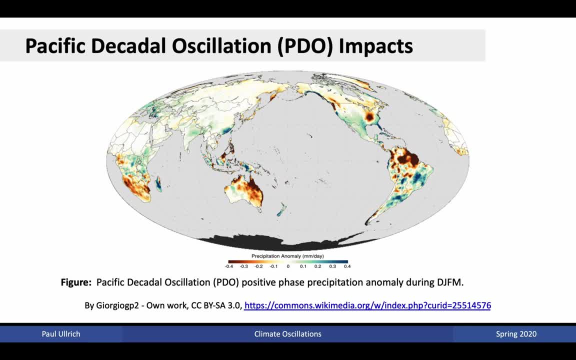 oscillation. During the positive mode we see more of the Pacific decadal oscillation and the Pacific decadal oscillation is typically much wetter conditions occurring along the coast of Alaska but drier conditions occurring in the Pacific Northwest. In California we see typically wetter conditions associated with the 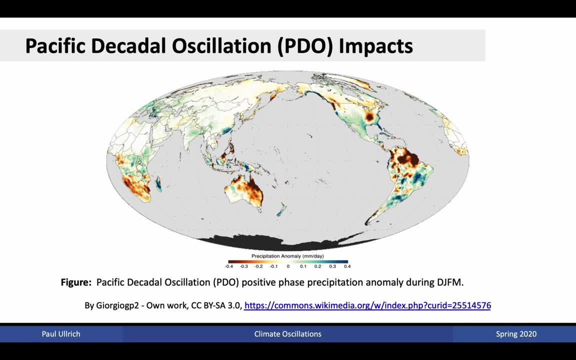 positive mode. This has to do with how this positive mode is impacting the geostrophic flow and thus the storm track in the vicinity of the eastern Pacific Ocean. However, we again see some widespread impacts in the precipitation because of this shift in the polarity of Pacific Ocean. 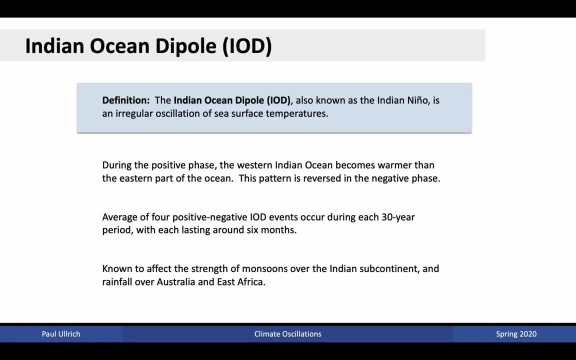 sea surface temperatures. The last pattern we'll consider in this lecture is the Indian Ocean Dipole, also called the IOD. This is also known as the Indian Nino because it is very closely associated with the El Nino. It's the Indian Ocean pair essentially to the El Nino. This is an 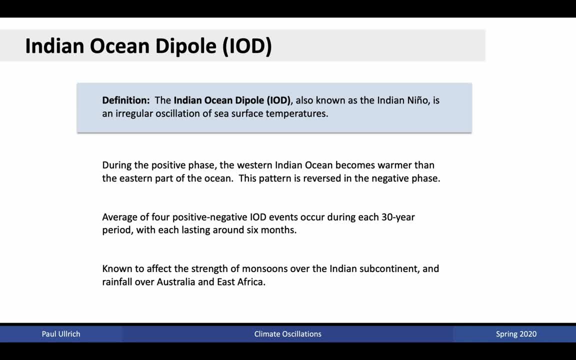 irregular oscillation of sea surface temperatures that occurs in the Indian Ocean. During the positive phase, the western Indian Ocean becomes warmer than the eastern part of the ocean. This pattern is reversed in the negative phase. There is an average of four positive-negative IOD events that occur during each 30-year period. 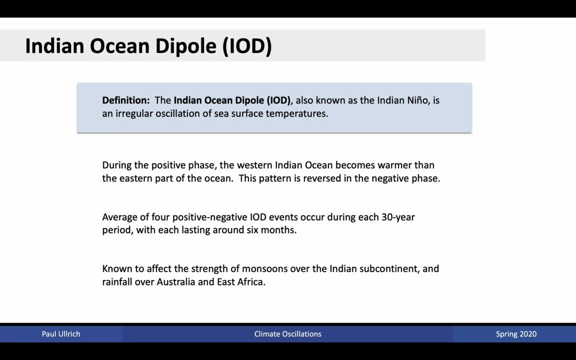 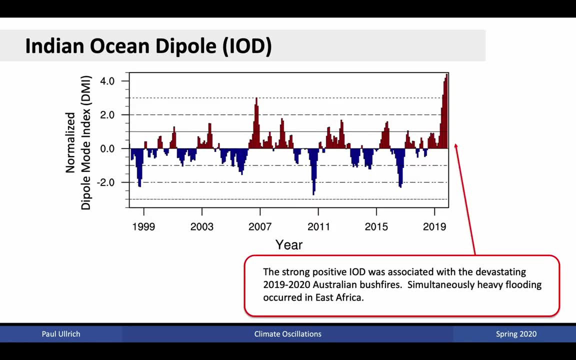 with each of the events lasting around six months. The IOD is known to affect the strength of monsoons over the Indian subcontinent, as well as rainfall over Australia and East Africa. Here we see the dipole mode index, which is used to quantify the strength of the Indian Ocean. 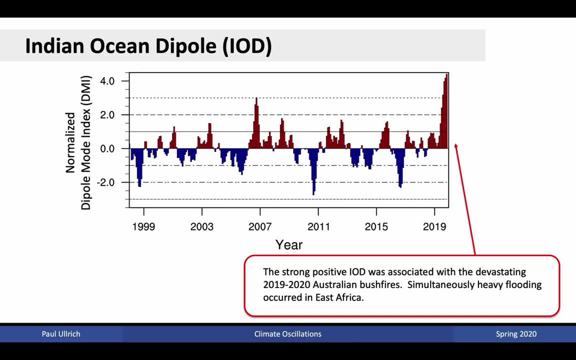 Dipole. It is equal to the Indian Ocean temperature in the western Indian Ocean, minus the temperature in the eastern Indian Ocean. Thus the indian ocean temperature is equal to the indian ocean temperature Plus. large positive values are associated with warmer temperatures in the West Indian. 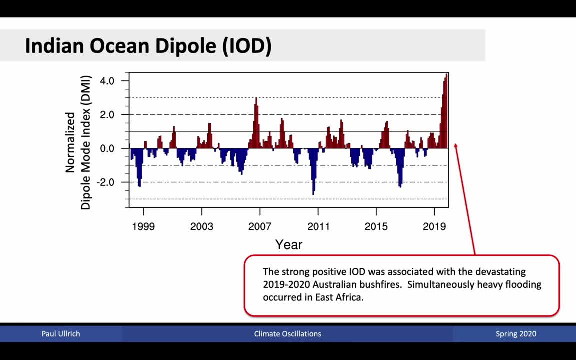 Ocean, and negative values are associated with warmer temperatures in the East Indian Ocean. Over the recent 2019 through 2020 season, the Indian Ocean experienced some of its largest values of the Dipole Mode Index. This was again associated with very warm temperatures in the Western Indian Ocean. 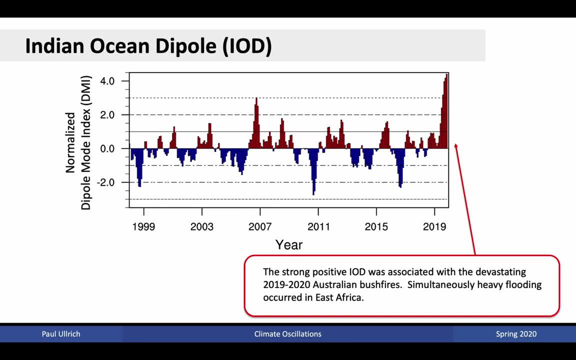 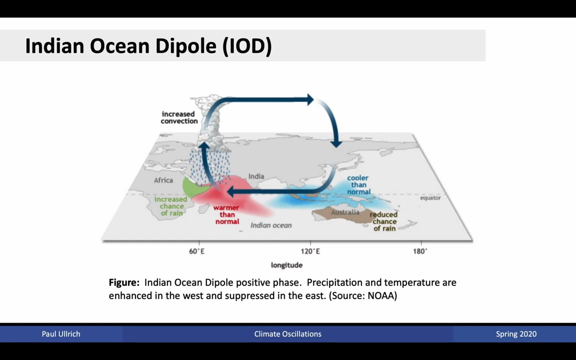 During this time, the suppressed precipitation that then occurred over Australia contributed to the devastating Australian bushfires that burned over this season. Simultaneously, heavy flooding occurred in East Africa, where warmer sea surface temperatures then contributed to increased convection and precipitation. Here's a depiction of what occurs during an Indian Ocean dipole positive phase. 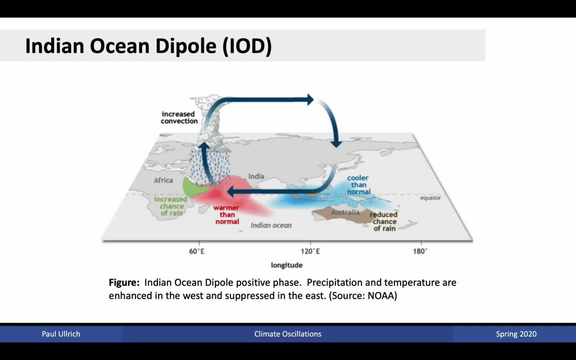 A large-scale circulation gets set up associated with these warmer conditions in the West Indian Ocean. Because the underlying sea surface temperatures are warm, they produce convection that dominates this region. A circulation then gets set up so that the air that gets convected upwards gets propagated. 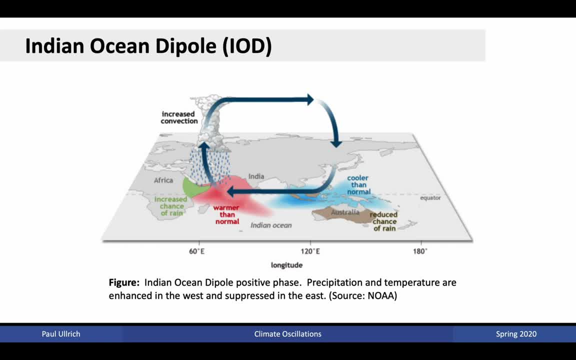 eastwards along the equator and then sinks over the eastern edge of the Indian Ocean. This sinking motion or subsidence then suppresses precipitation in this region and is associated with cooler sea surface temperatures. This circulation, set up during this positive phase, then contributes to an increased chance.